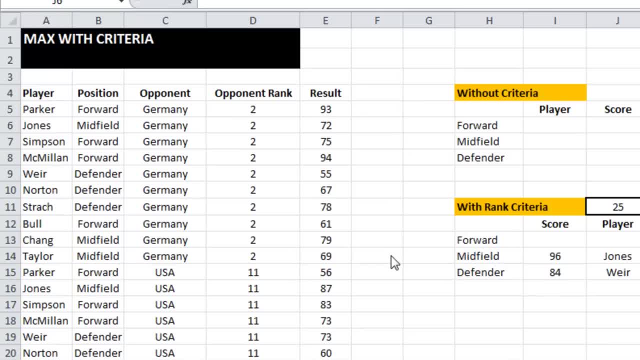 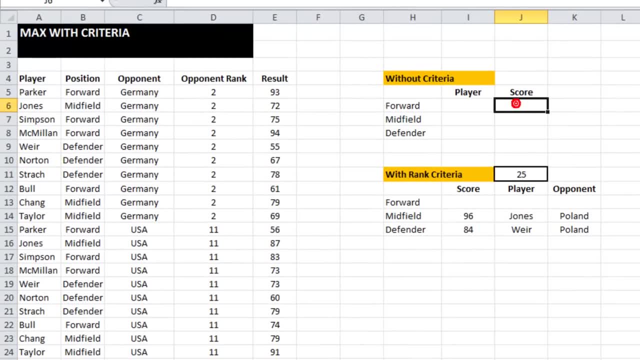 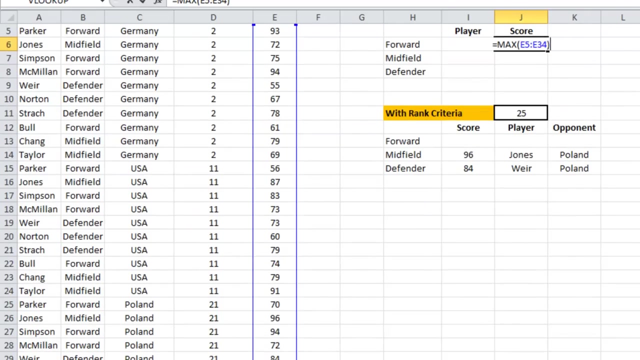 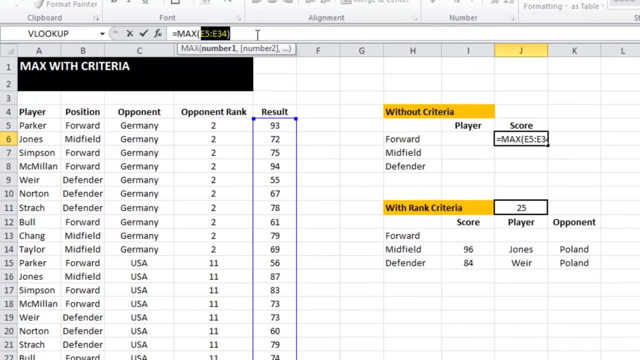 Unfortunately we can't do that for max, so we're going to write an array formula to accomplish the same thing. So what we've got here is: I'll do the score first. I want to find out the maximum result in this list, So that's relatively easy to do, but I want to find only. 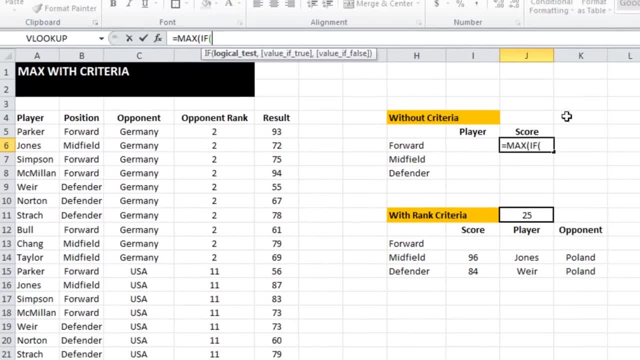 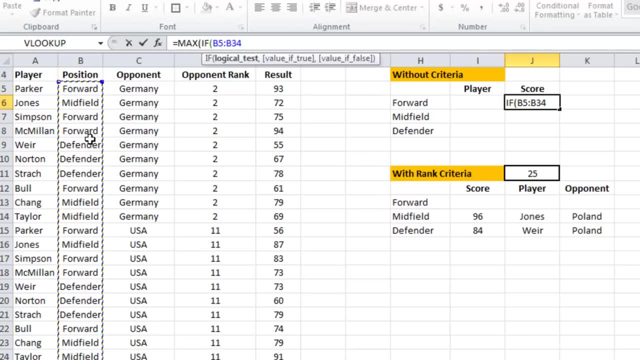 the maximum if I get the maximum result. So I'm going to write an array formula to they were a forward. so I need to put an if equation inside the max. I want to lock that, I also want to lock that. so basically what that's saying is: if the 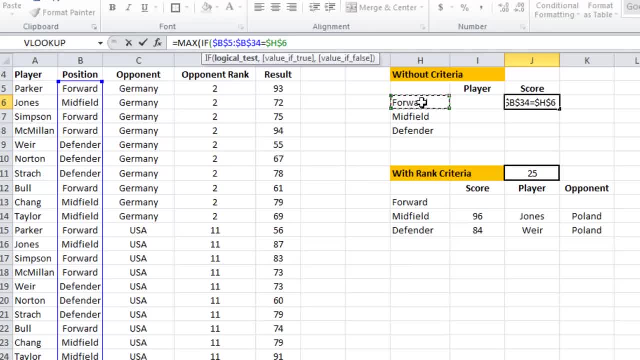 position in column B is equal to a forward, then I want you to include the result in colony, and you know that I'm using dollar signs throughout this, because it's really important that I can drag this down a little bit later. so I've closed that off now and unfortunately this isn't a normal. 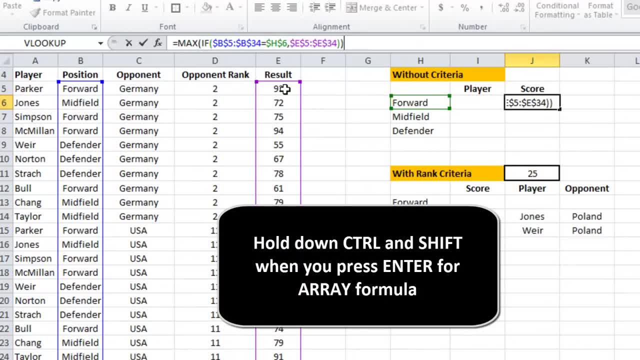 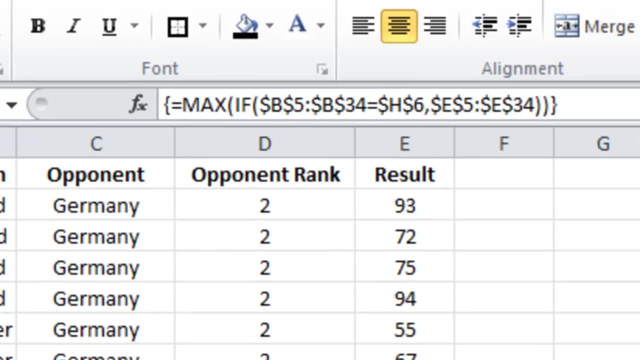 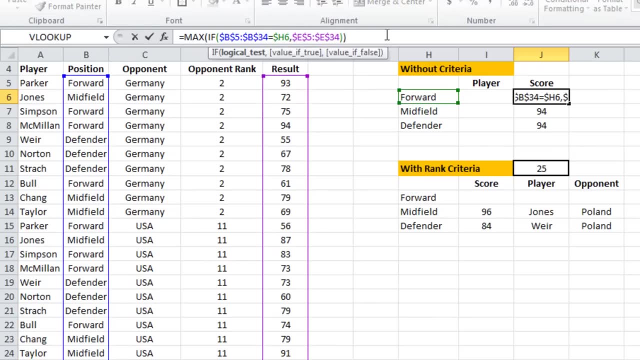 formula. I can't just hit enter, I have to go control, shift, enter and you can see an array formula puts a curly bracket around the beginning and the end of the formula. just made a little mistake there. I need to take that dollar sign out so that when 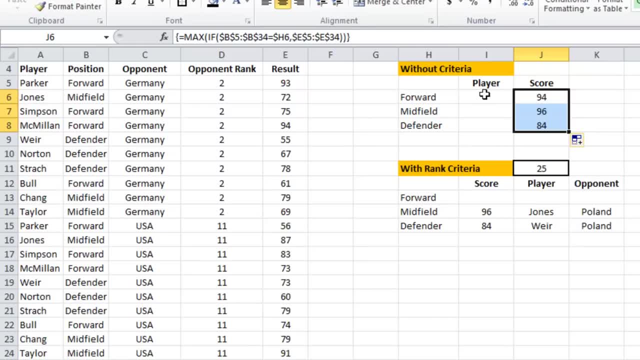 it copies down. it changes from midfield to defender. so that's great. I've found out what the best score for a forward or a midfielder or a defender is. but I would also be good if I could find out which player got that score. so first thing, I 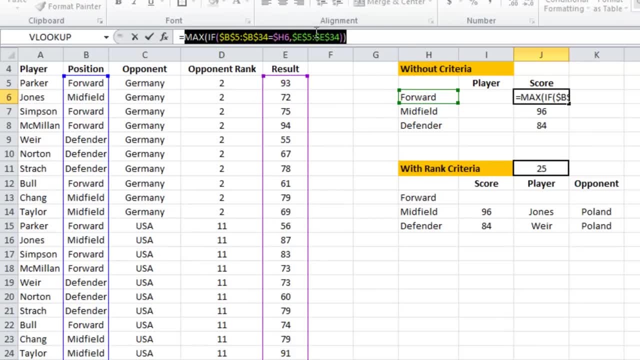 want to do, just to make it easy for myself, because I want to scoop out that answer there. I want to use an index equation. what do I want to find? I want to find the player name lock that and I want to use the match equation to find. 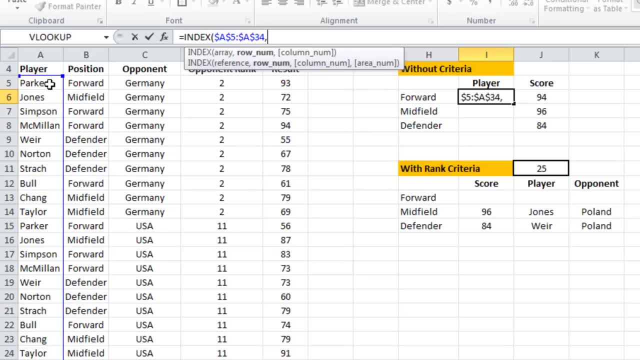 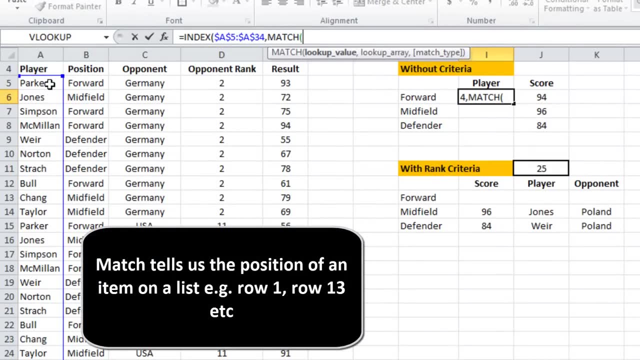 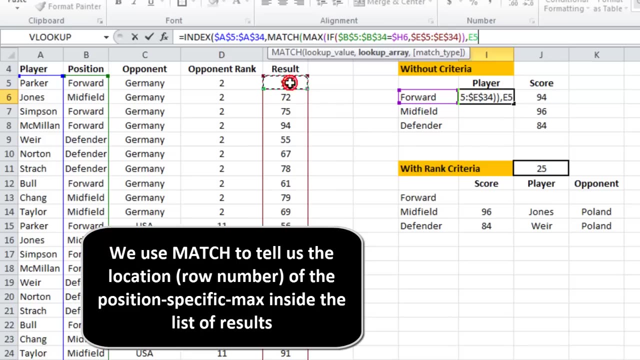 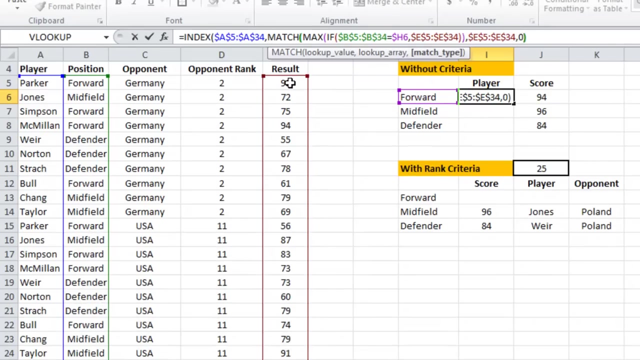 which row number that player name is in, based upon the max score. what do I want? to look up whatever was attached to them. back again, I'm going to drag this box up in here and I'm going to do a simple and I'll find that the person that has the maximum score for a forward 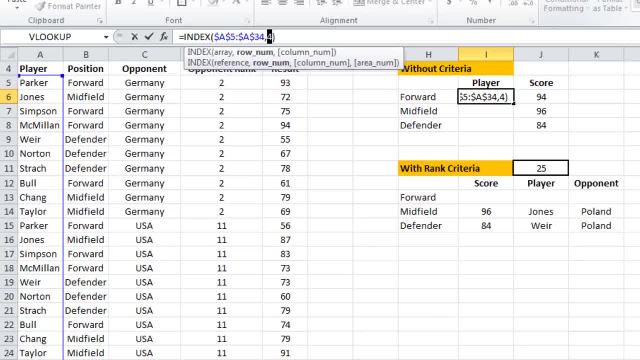 is in the fourth row of our grid. Because there's an array inside this index function, I have to use Control-Shift-Enter again. If I drag that down, what we'll find is things change a little bit. So to test that this works, I'm just going to change that to 97.. 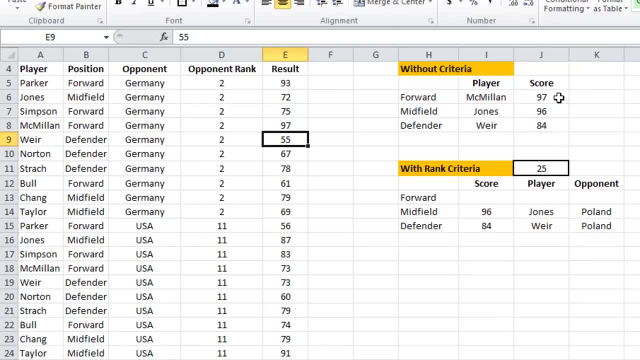 And see what happens. That's great. That updates- And I'm also going to change that- And that updates as well, So that's looking good. So, with a single criteria, we've just written a formula that will find the maximum score for each particular subgroup. 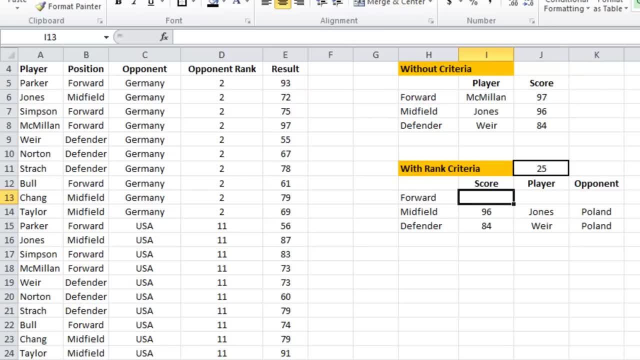 What I want to do is extend it a little bit further and use a second criteria. It's not that much different, but as soon as you start nesting functions inside another, it does become a little bit of a challenge. So I'm just going to write it from scratch. 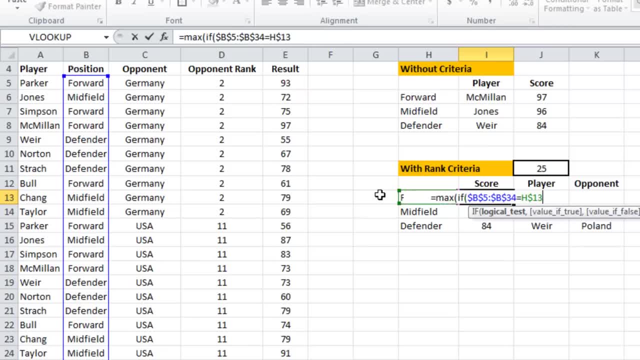 Sometimes you have to use your arrow keys to be able to see the parts of the cell that you want to see, So I'm going to go straight into my second if equation. So if the first if is true, then go straight into the next if. 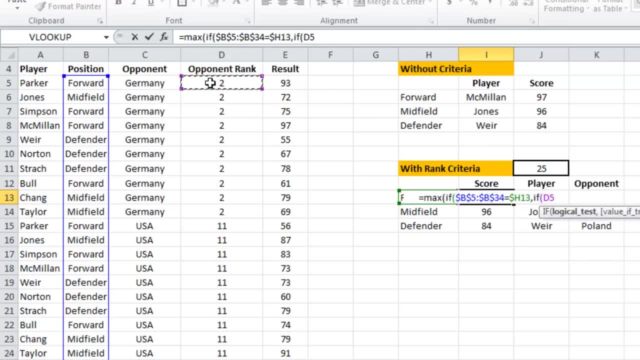 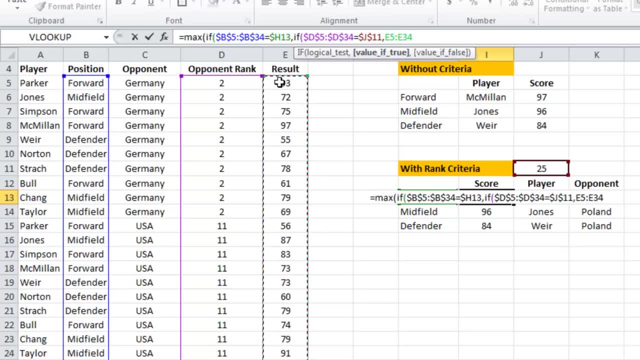 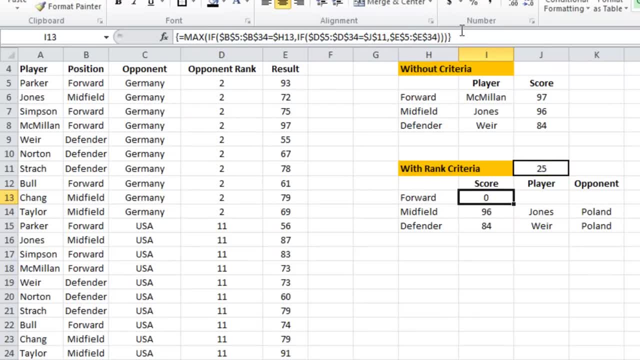 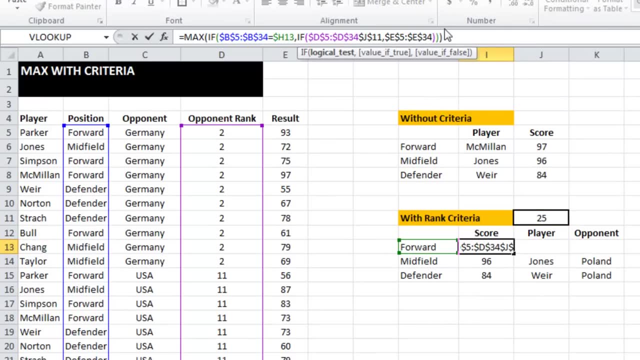 Control shift- enter. I just made a little mistake here. I shouldn't have put equal to j11. I should have put is less than j11.. Now if I just drag that down, what I'll find is that I've got some new scores out there, and so if I look for 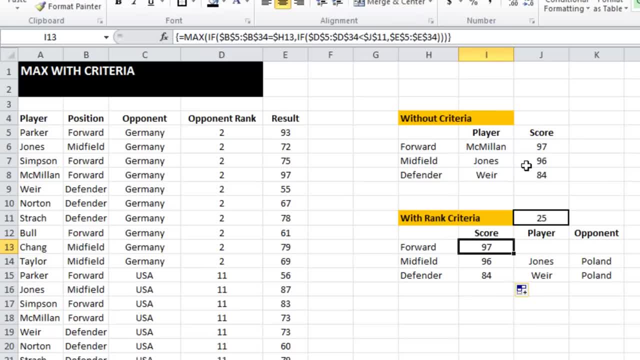 forward again. we've got the same as up above there, Macmillan. what I want to do now to assess whether this has worked or not. let's just change that, and here we get a change. the best midfield score up here and that's worked out. so that's. 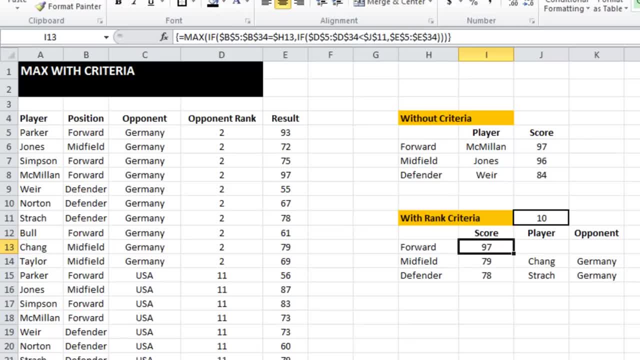 great. so we've got two ifs inside one max array formula, so we're going to use the same logic to pull out who the player was and who the opponent was in this particular instance. so I will select that, taking away the equal sign. so what I tend to do is I just put my 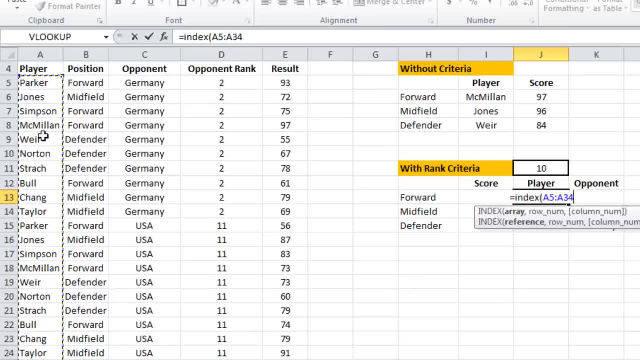 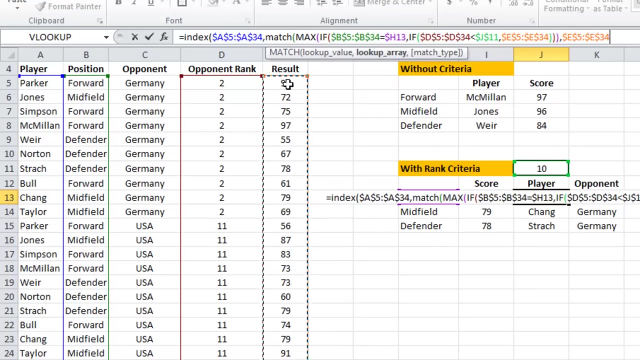 I just put my cursor in the first value and I had ctrl, shift down, arrow and then f4 paste my array, and I should really just have to fill in the blanks here, keeping my if fours all the way through, making it an exact match and then closing it off. so that's. 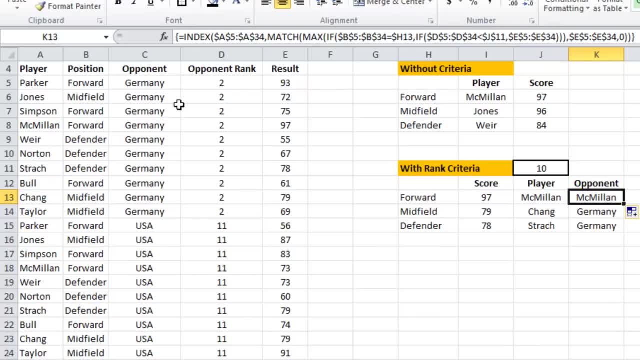 good, I'll drag that across and instead of wanting to you do an index of the name, I'll just pull that across to the opponent and go to ctrl shift a个 and drag that down. If I change this to 15, it allows the second games data to be included. 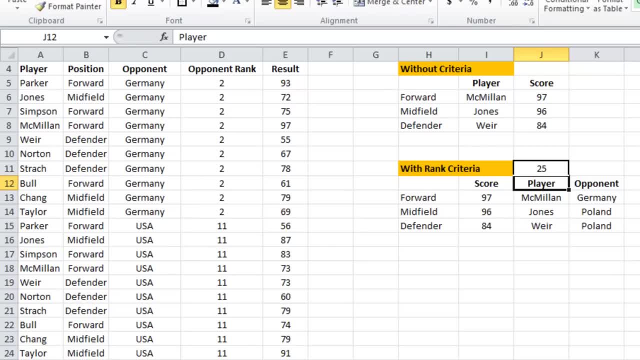 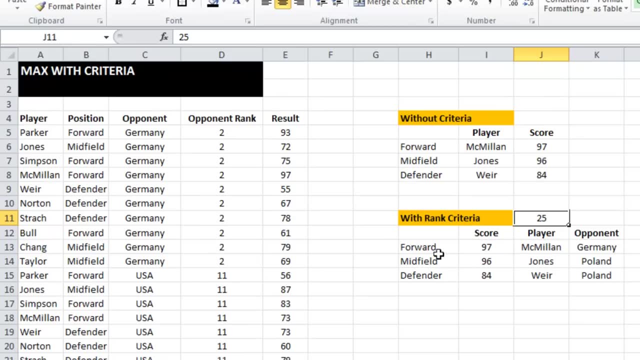 in the criteria. If I change it to 25, it allows the third games data to be included in the criteria. So that's working A max if equation quite useful a little bit gnarly. What you need to do is understand how some of these formula work, and to do so you can.